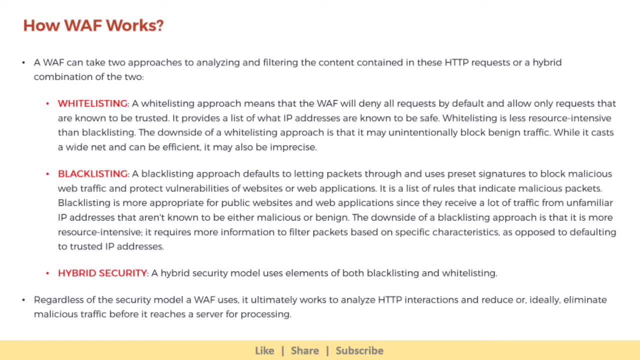 HTTP requests or a hybrid combination of the two. A whitelisting approach means that the WAF will deny all requests by default and allow only requests that are known to be trusted. It provides a list of what IP addresses are known to be safe. 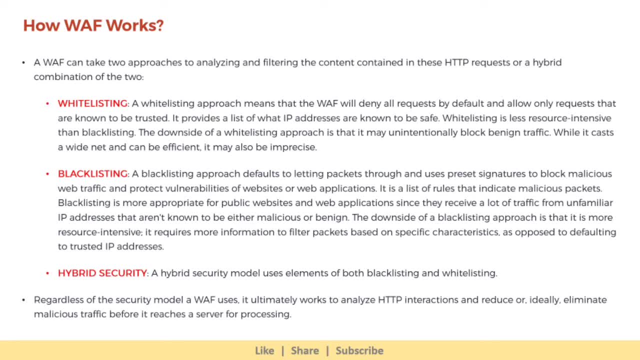 Whitelisting is less resource-intensive than blacklisting. The downside of a whitelisting approach is that it may unintentionally block benign traffic. While it casts a wide net and can be efficient, it may also be a risk-free approach. While it casts a wide net and can be efficient, it may also be a risk-free approach. 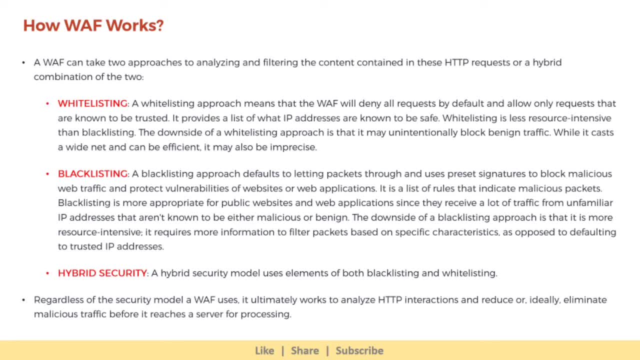 While it casts a wide net and can be efficient, it may also be a risk-free approach. While it casts a wide net and can be efficient, it may also be imprecise. On the other hand, a blacklisting approach defaults to letting packets through and uses 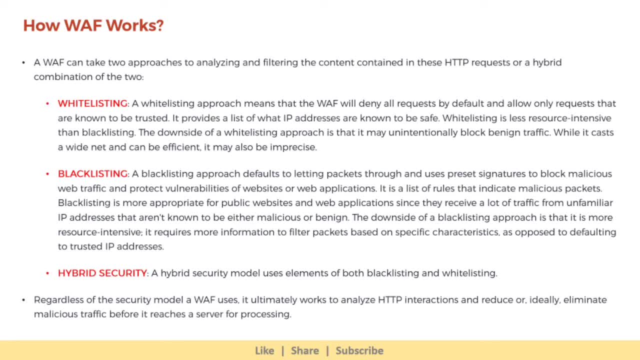 preset signatures to block malicious web traffic and protect vulnerabilities of websites or web applications. It is a list of rules that indicate malicious packets. Blacklisting is more appropriate for public websites and web applications, since they receive a lot of traffic from unfamiliar IP addresses that aren't known to be either malicious. 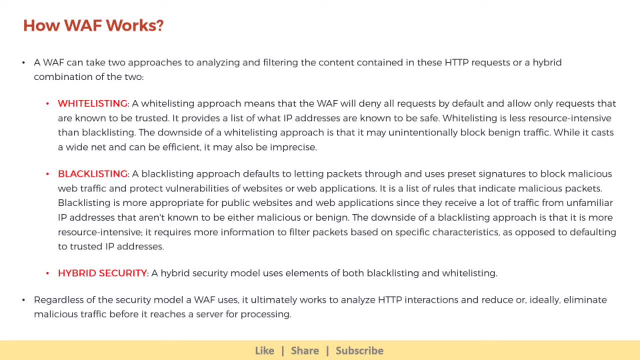 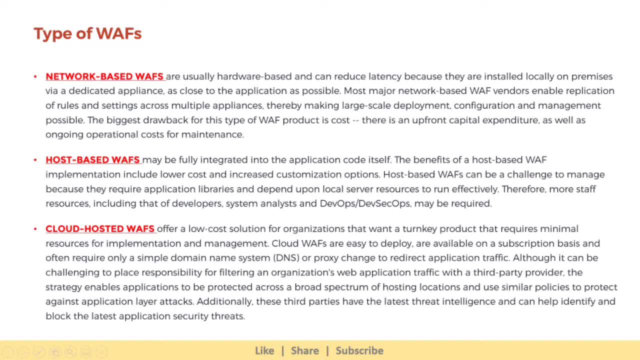 The downside of a blacklisting approach is that it may also be imprecise. biggest drawback for this type of WAF product is cost, that is, there is an upfront capital expenditure as well as ongoing operational costs for maintenance. Host-based WAFS may be fully. 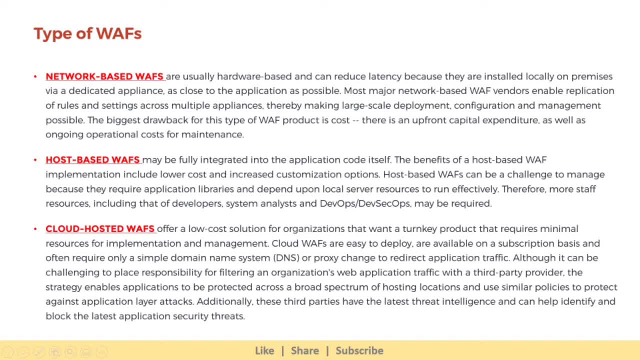 integrated into the application code itself. The benefits of a host-based WAF implementation include lower cost and increased customization options. Host-based WAFs can be a challenge to manage because they require application libraries and depend upon local server resources to run effectively. Therefore, more staff resources, including that of developers, system analysts. 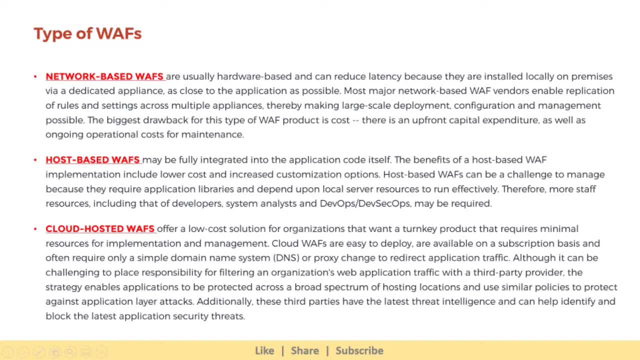 and DevOps or DevSecretaryOps may be required. Cloud-hosted WAFS offer a low-cost solution for organizations that want a turnkey product that requires minimal resources for implementation and management. Cloud WAFS are easy to deploy, are available on a subscription basis and often 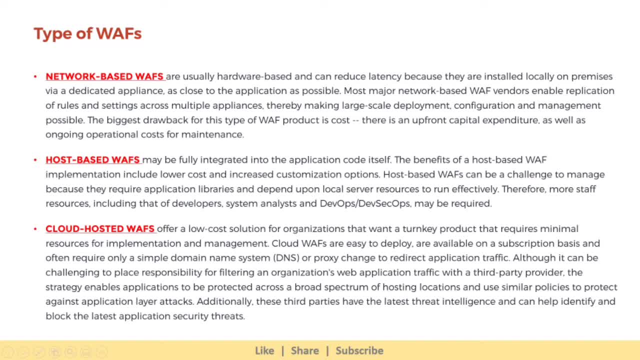 require only a simple domain name system or proxy change to redirect application traffic. Although it can be challenging to place responsibility for filtering an organization's web application traffic with a third-party provider, the strategy enables applications to be protected across a broad spectrum of hosting locations and use similar policies. 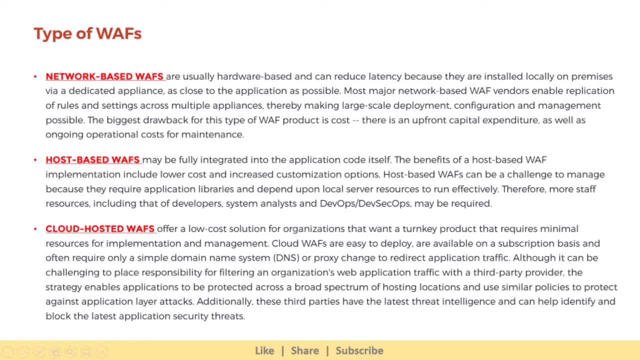 to protect against application layer attacks. Additionally, these third-parties have the latest threat intelligence and can help identify and block the latest application's security threats. A WAF has an advantage over traditional firewalls because it also provides better accountability over conditions with specific security measures, Whether it concerns a certain 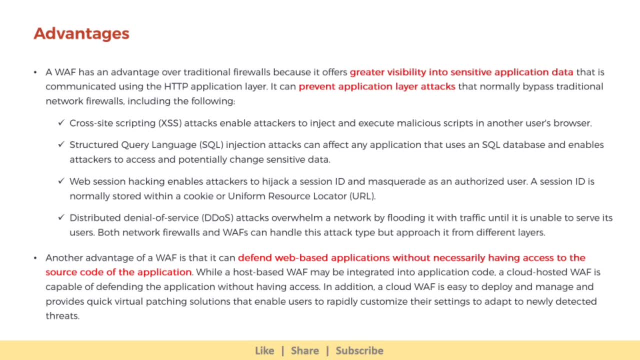 offers greater visibility into sensitive application data that is communicated using the HTTP application layer. It can prevent application layer attacks that normally bypass traditional network firewalls, including the following: cross-site scripting attacks enable attackers to inject and execute malicious scripts in another user's browser. Structured query. 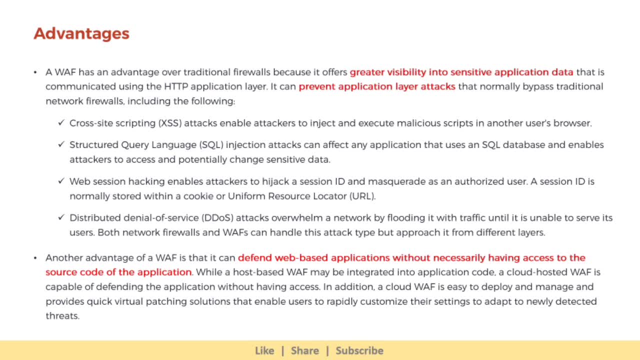 language injection attacks can affect any application that uses an SQL database and enables attackers to access and potentially change sensitive data. Web session hacking enables attackers to hijack a session ID and masquerade as an authorized user. A session ID is normally stored within a cookie or uniform resource locator. Distributed denial-of-service. 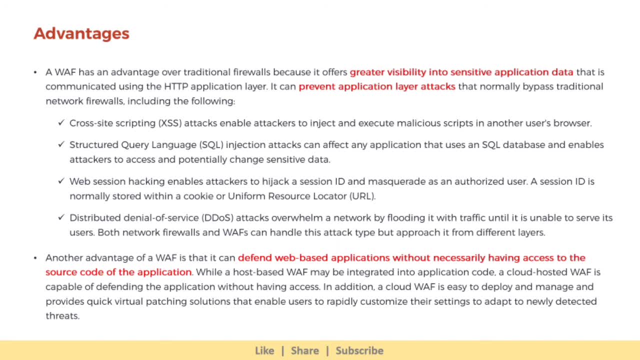 attacks overwhelm a network by flooding it with traffic until it is unable to serve its users. Both network firewalls and WAFs can handle this attack type, but approach it from different layers. Another advantage of web session hacking is that it can be used in a variety of ways. 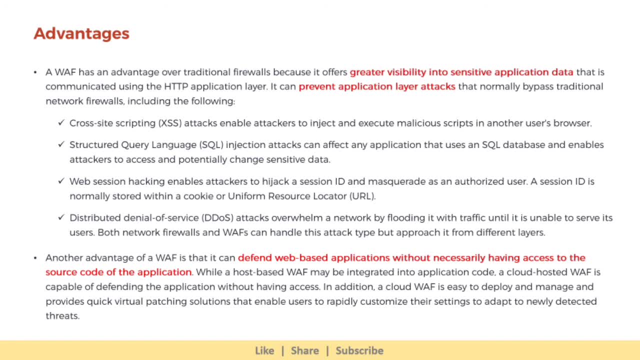 The advantage of a WAF is that it can defend web-based applications without necessarily having access to the source code of the application. While a host-based WAF may be integrated into application code, a cloud-hosted WAF is capable of defending the application without having access. 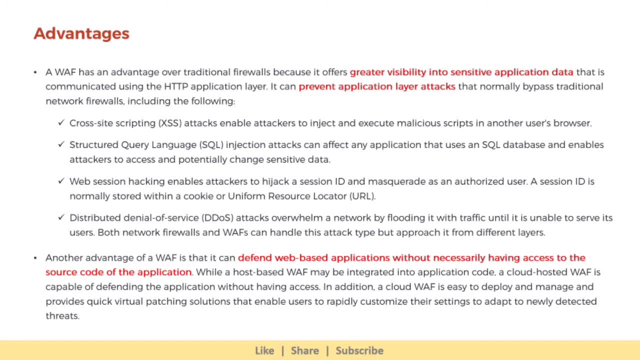 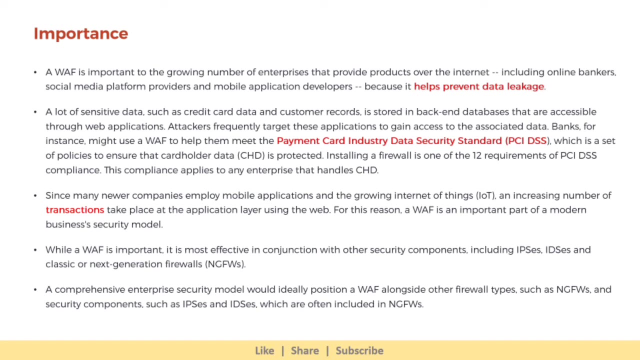 In addition, a cloud WAF is easy to deploy and manage and provides quick virtual patching solutions that enable users to rapidly customize their settings to adapt to newly detected threats. A WAF is important to the growing number of enterprises that provide products over the internet, including online bankers, social media. 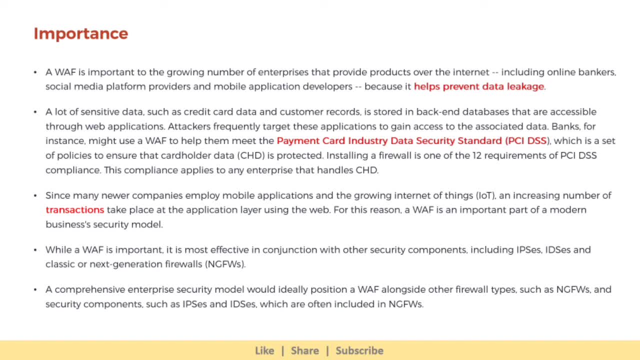 platform providers and mobile application developers, because it helps prevent data leakage. A lot of sensitive data, such as credit card data and customer records, is stored in back-end databases that are accessible through web applications. Attackers frequently target these applications to gain access to the associated data Banks, for instance, might use a WAF to help. 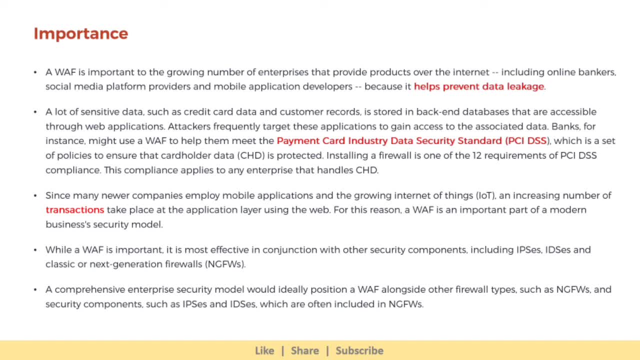 them meet the Payment Card Industry Data Security standard, which is a set of policies to ensure that cardholder data is protected. Installing a firewall is one of the 12 requirements of PCI DSS compliance. This compliance applies to any enterprise that handles cardholder data. 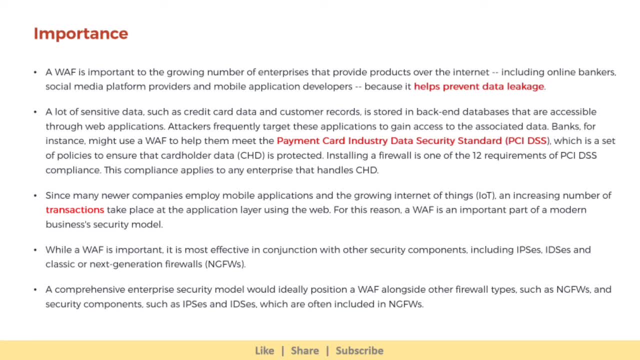 Since many newer companies employ mobile applications and the growing internet of things, an increasing number of transactions take place at the application layer using the web. For this reason, a WAF… is an important part of a modern business's security model. While a WAF is important, it is most effective in conjunction with other security components, including IPS, IDS and classic or next-generation firewalls. A comprehensive enterprise security model would ideally position a WAF alongside other firewall types such as NGFWs and security components such as IPS and IDS, which are often included in next-generation firewall. 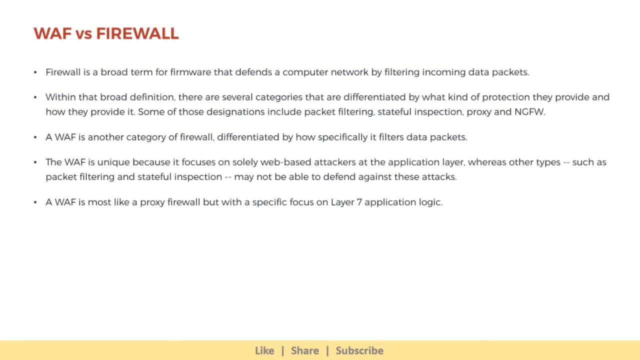 Let's now compare WAF and firewall. Firewall is a broad term for firmware that defends a computer network by filtering incoming data packets. Within that broad definition, there are several categories that are differentiated by what kind of protection they provide and how they provide it. Some of those designations include packet filtering, stateful inspection. 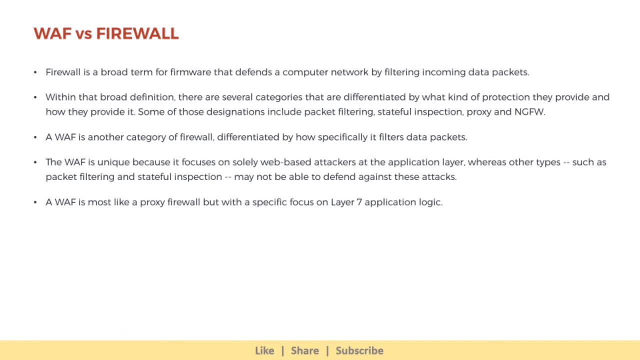 proxy and next-generation firewall. A WAF is another category of firewall, differentiated by how it is used. A WAF is a type of firewall that is used to filter data packets. The WAF is unique because it focuses on solely web-based attackers. at the